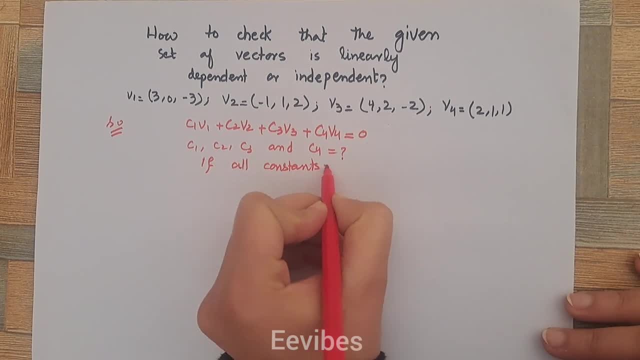 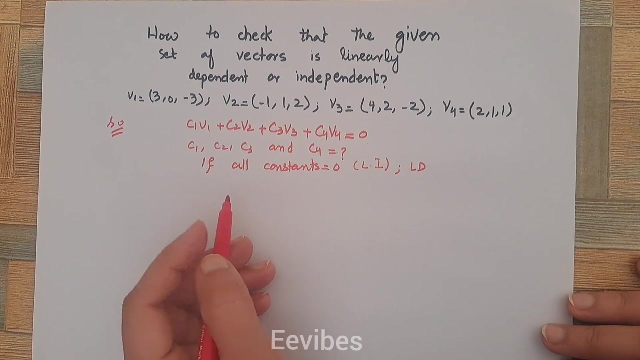 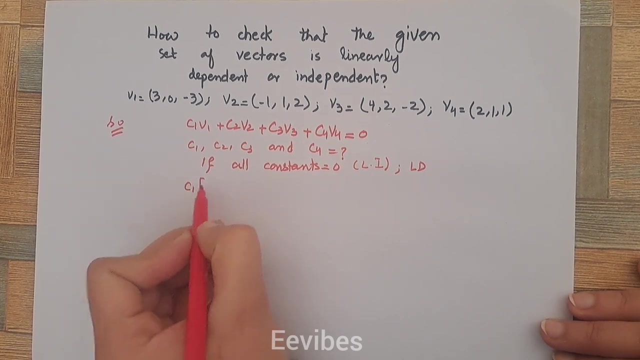 then the vectors will be linearly independent. fine, otherwise linearly dependent. If any of the constants comes out to be some constant, then we are trying to find the values of these constants. So let's start solving it. So I will write it as c1 and substitute the value of v1, which 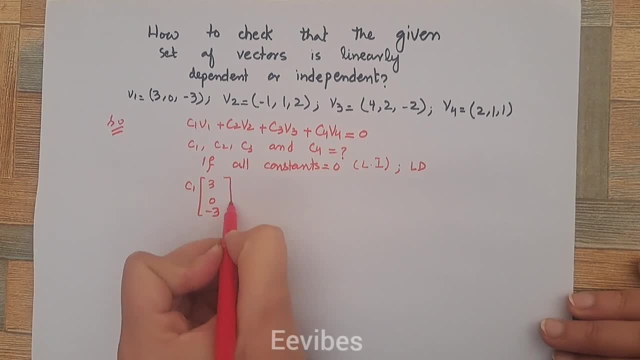 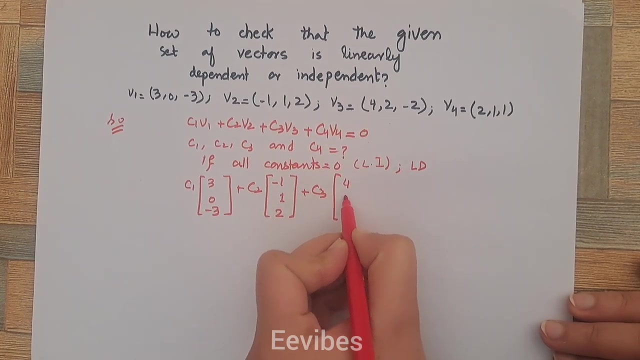 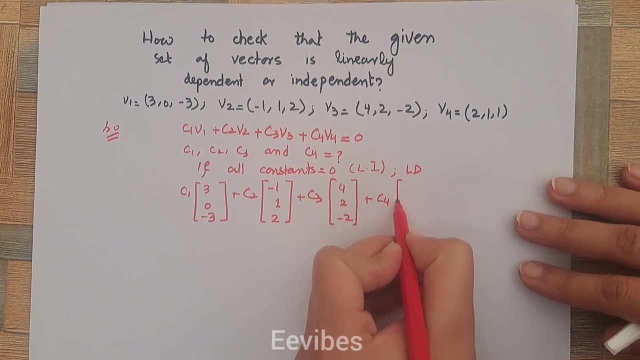 is equal to 3, 0 minus 3 plus c2, and then put the value of v2, which is equal to minus 1, 1 and 2, then plus c3 and v3 is 4, 2 minus 2. alright, Then the last vector is v4, whose components are 2, 1 and 1.. On the right hand side we have 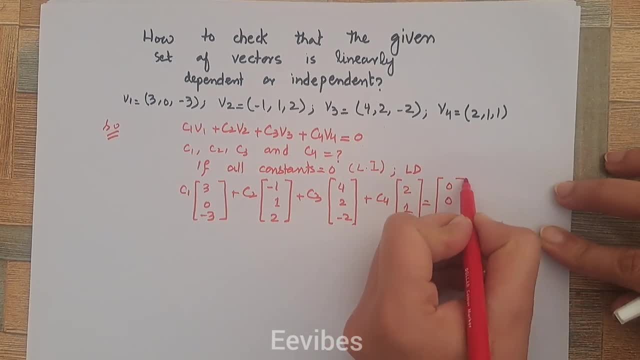 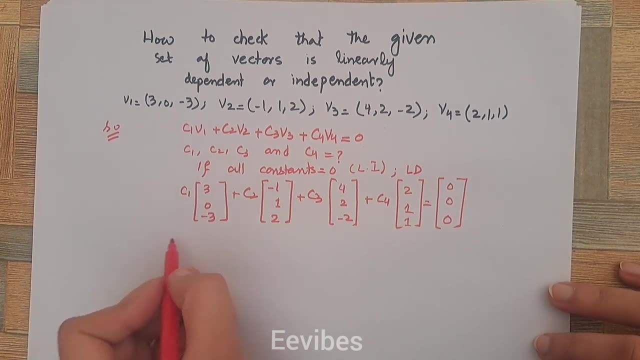 to write the 0 vector and its entries will be equal to the number of rows in the column vectors. fine, Now the next step is to develop or construct the linear system equation. So this becomes 3 times of c1 minus c2 plus 4 times of c3 minus c4 minus c5 minus c6 minus. 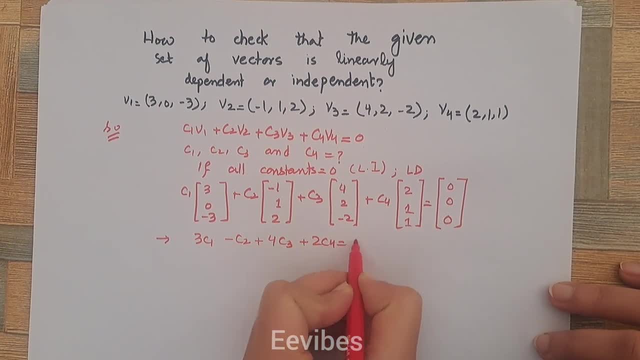 2 times of c3 plus 2 times of c4 should be equal to 0.. Similarly, 0 times of c1 plus c2 plus 2 c3, then plus c4, should be equal to 0, while the last equation is: minus 3 c1 plus 2 c2, minus 2 c3 plus. 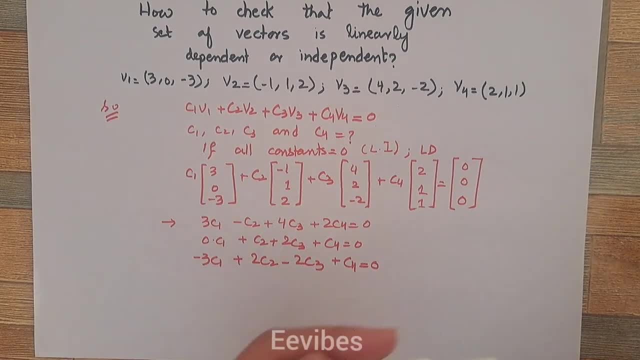 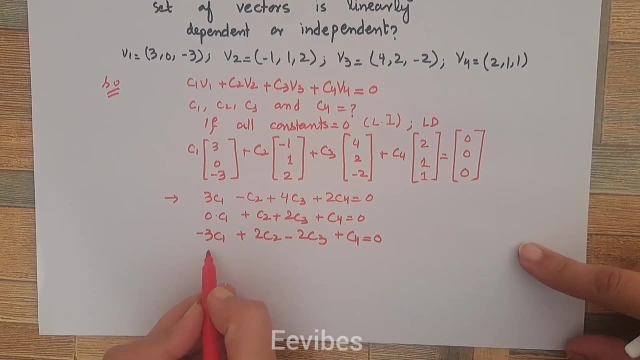 c4 is equal to 0.. Okay, once you are done with writing this system of the linear equations, then solve it by applying the Gauss elimination method, and for that you need to write this system of equations in the form of the augmented matrix which can be constructed from the minus. 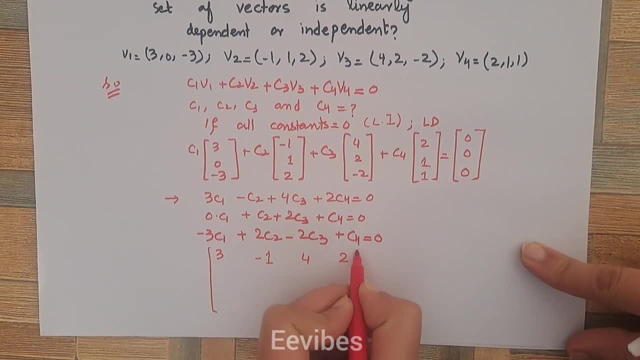 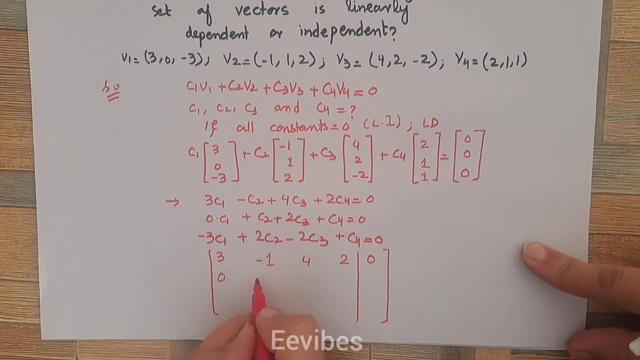 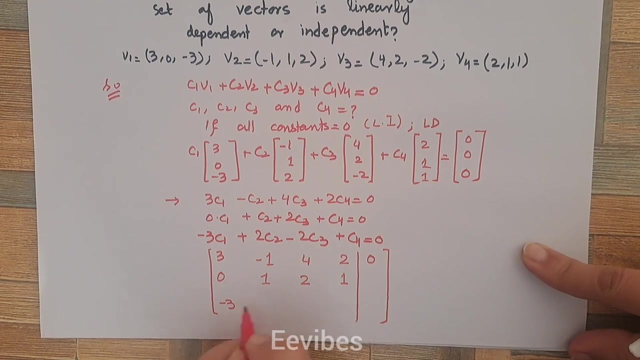 3 minus 1, 4 and 2, while on the right hand side we will write the b vector, which is 0 in this case, because this is a homogeneous system. Fine, we have 0, then 1, the coefficient of c3 is 2, the coefficient of c4 is 1 and then minus. 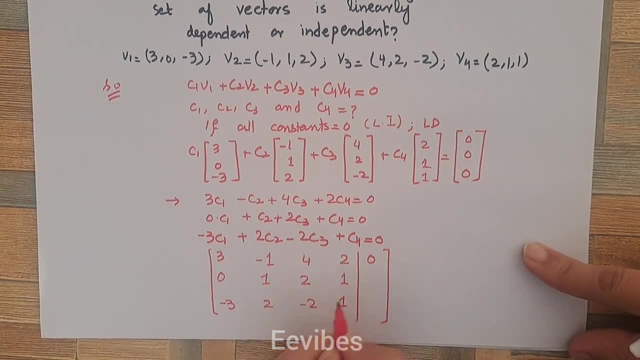 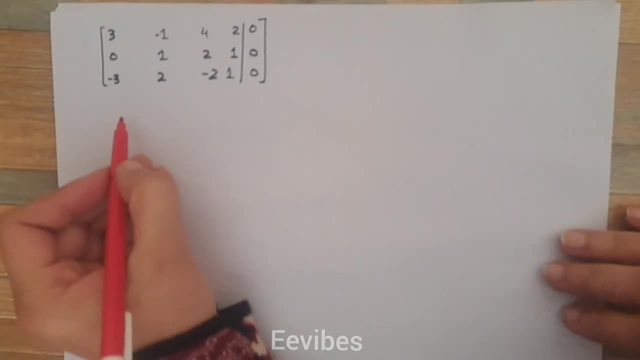 3. So we have 2 minus 2 and 1, and here we will have 0.. Okay, so in this matrix we can see that this is the pivot entry and according to the Gauss elimination we have to convert this matrix into the upper triangular matrix for that. 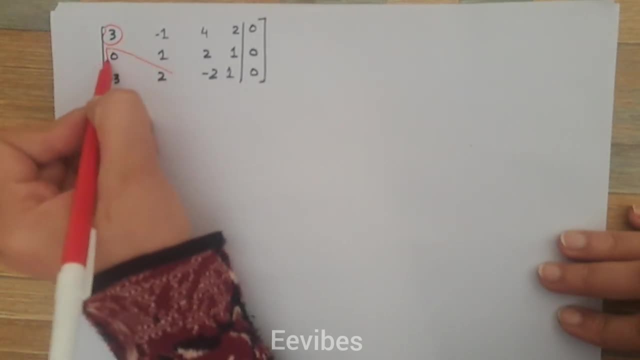 what we need to do. we need to make all these entries equal to 0, and this is our first pivot. so that's why we need to make this entry equal to 0 and for that I will perform the operation on R3. so the change will be made in R3, which is denoted by this tilted sign. 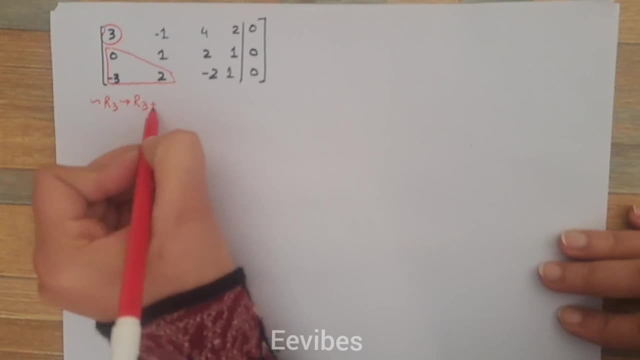 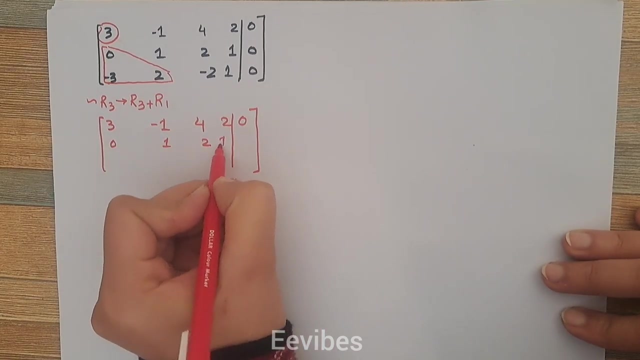 and according to this we will do that: R3 plus R1. fine, so let's just do it now. it becomes 3 minus 1, 4, 2, and here you will have 0, 0, 1, 2, 1, 0, and when you will perform the operation. 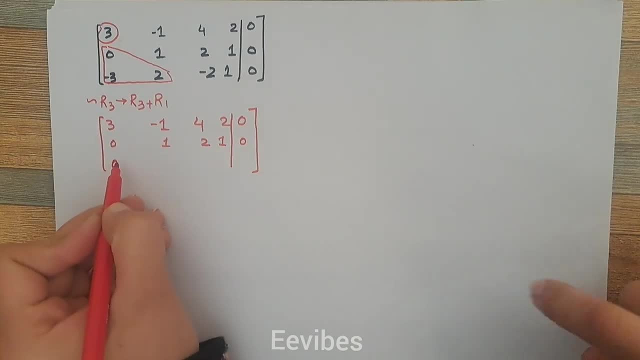 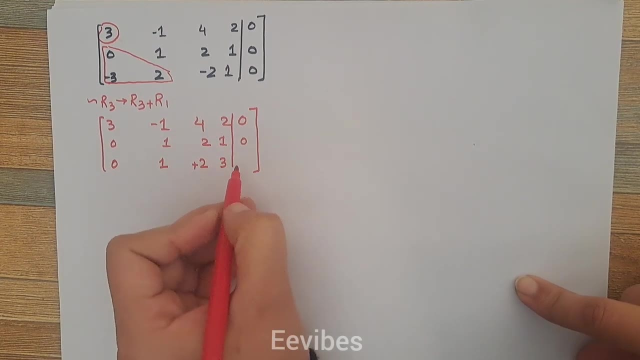 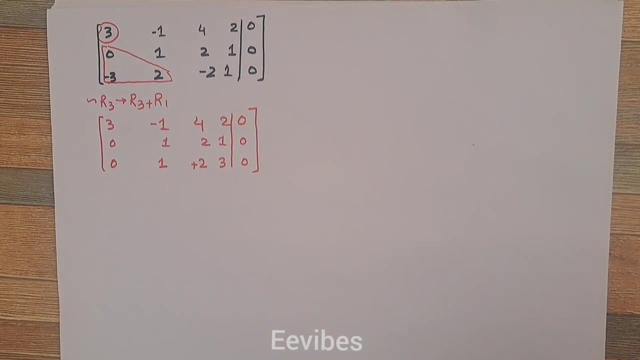 of R3 plus R1.. 2 minus 1 is 1,, 4 minus 2 is plus 2,, 2 plus 1 is 3, and here you will have 0. ok, Then in the second row, we can see that this is our pivot entry and we have to make all. 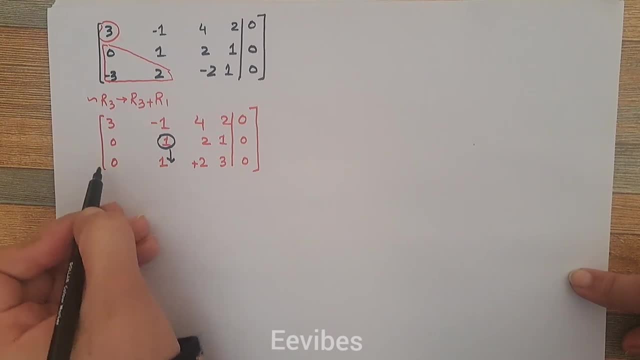 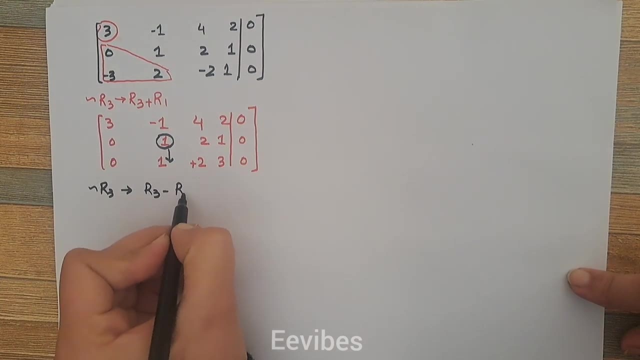 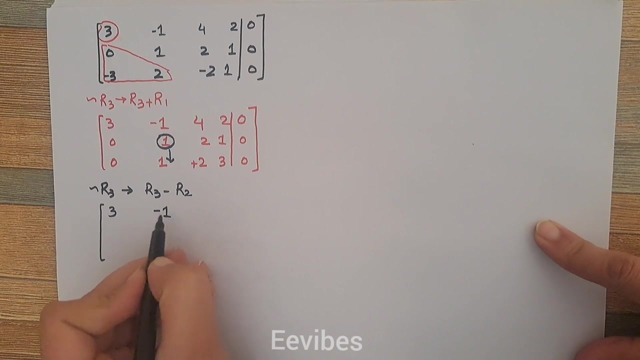 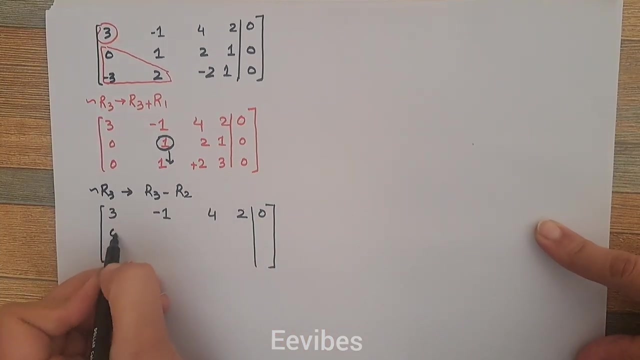 the entries below it equal to 0. So we need to make the change again in R3 and that will be R3 minus R2, simply fine. So let's apply this operation and look what we will get. So you will have 3 minus 1, 4, 2 and then 0, no change in R1, no change in R2, because 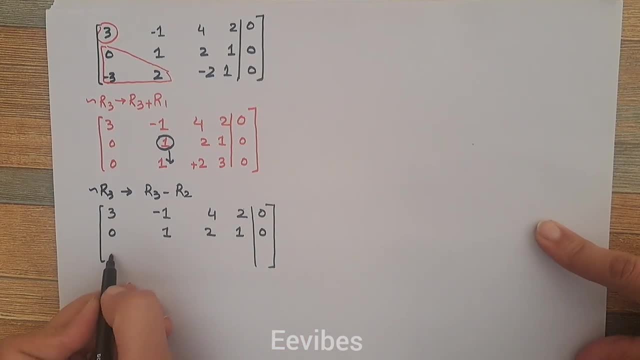 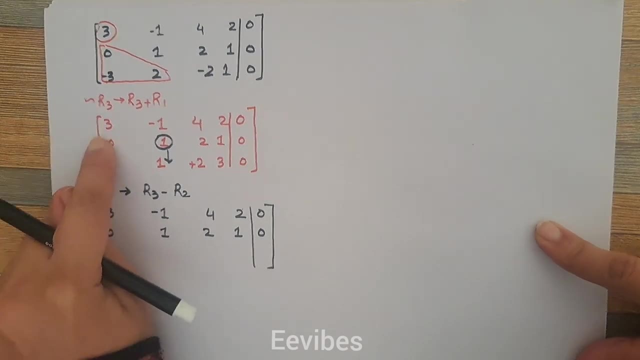 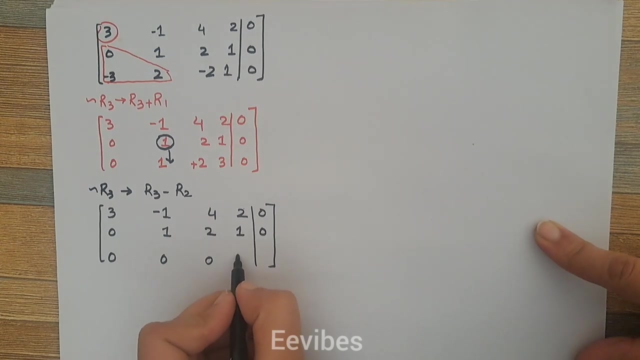 there is no operation applied. fine, but we will change the values of R3. why? Because the operation is performed on R3, which is R3 minus R2.. So 0 minus 0 is 0, 1 minus 1 is 0, 2 minus 2 is 0 and 3 minus 1 is equal to 2, while on 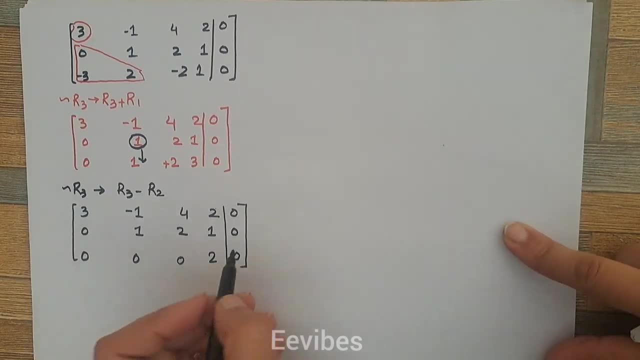 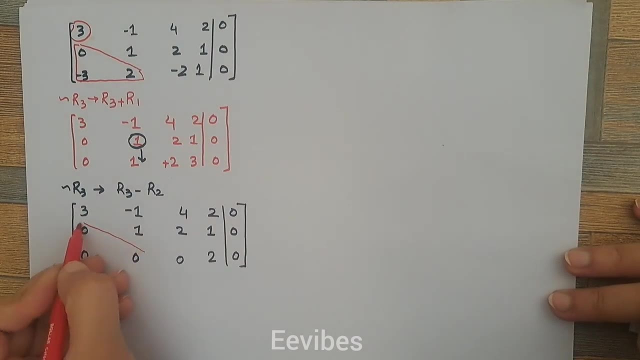 the right hand side, you will have 0 again. Now we can see this matrix has been converted into an upper triangular matrix. So we are done with applying the Gauss elimination. The next step is to perform the back substitution. If you remember that, these were the coefficients: 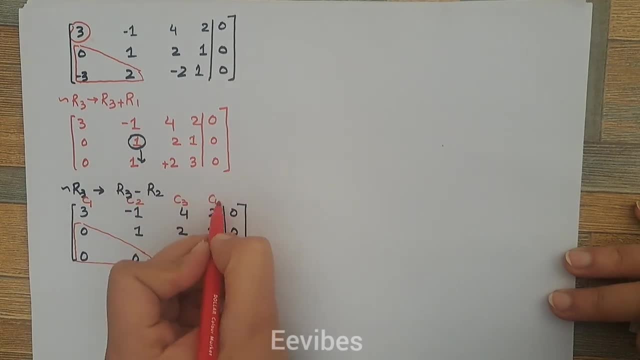 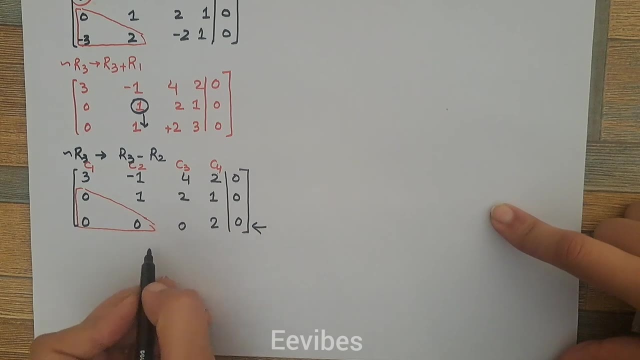 These are the coefficients of C1, C2, C3 and C4. fine, So we will now build, or reconstruct, the equations and we will start from the bottom. So we will have: 2 times of C4 is equal to 0.. 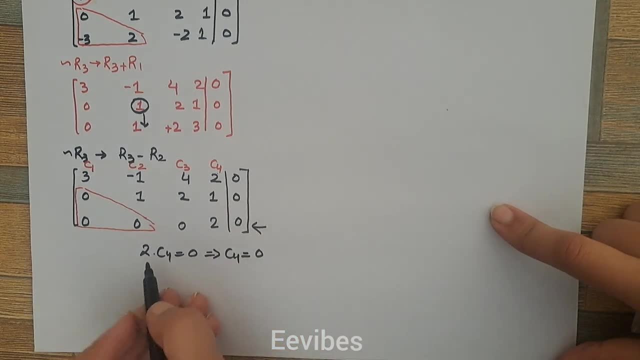 This implies C4 must be equal to 0, because 2 is some non-zero number, So it must be multiplied with a 0 in order to get the 0, in order to satisfy this equation. fine, The next equation will be C1. 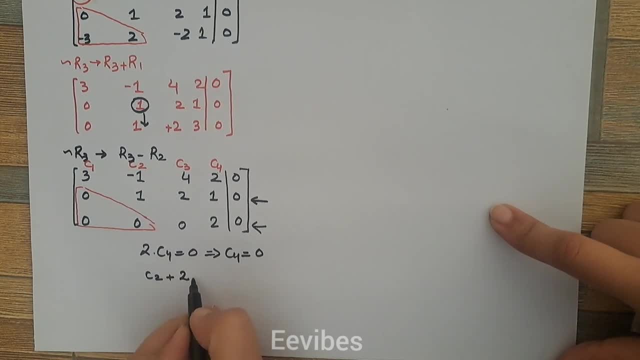 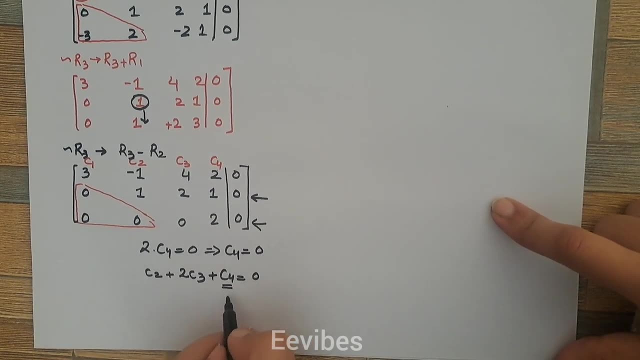 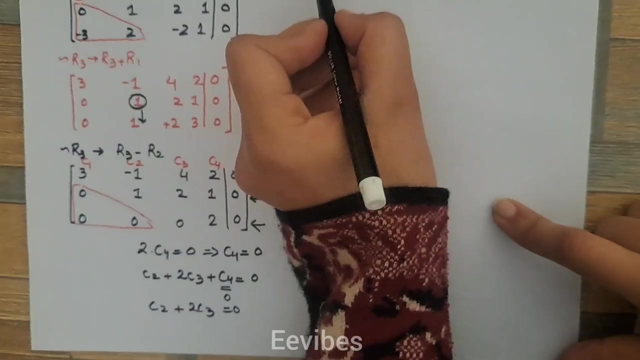 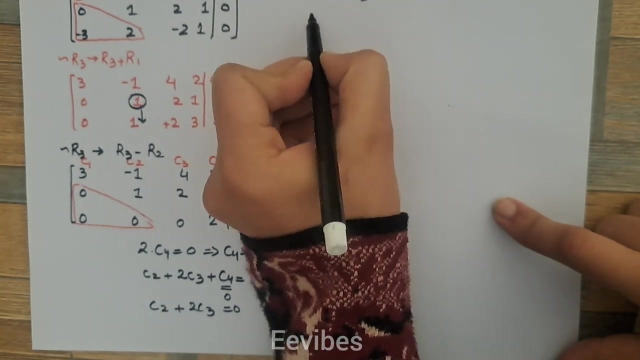 C2 plus 2 times of C3 plus C4 should be equal to 0.. Since C4 is 0, we will have C2 plus 2 times of C3 equal to 0, and from here we can write it as C2 is equal to minus 2 times of C3. 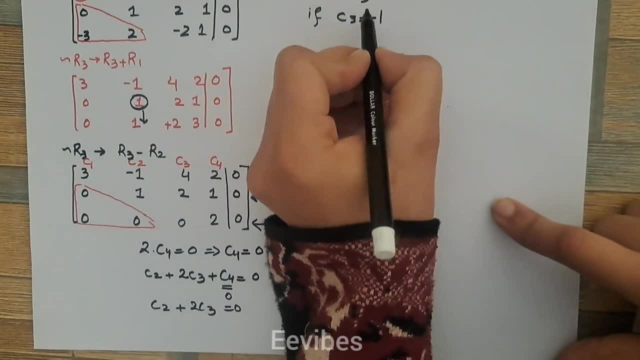 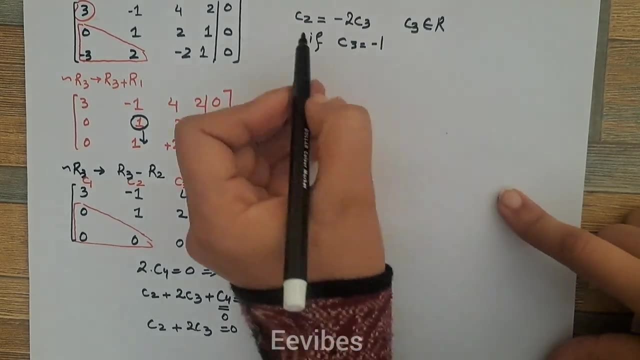 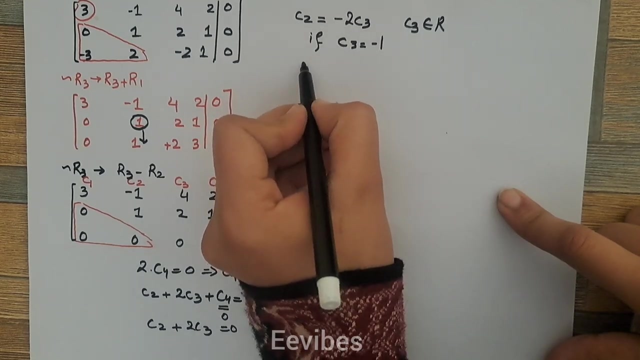 If I choose, C3 is equal to minus 1.. Why? Because C3 is a free variable. It can take any value from the set of real numbers. ok, So I have selected minus 1.. Why? because I want to eliminate this minus from here. 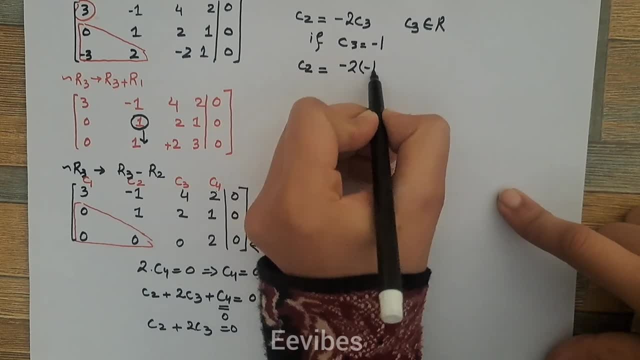 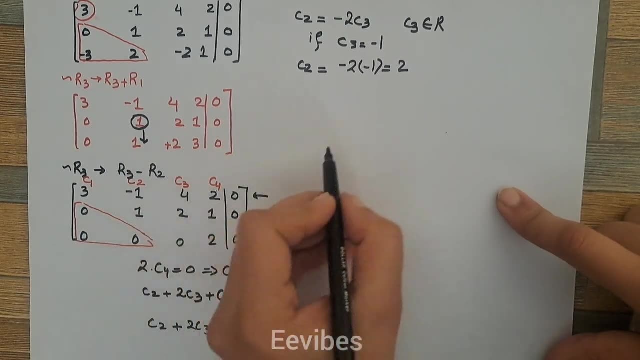 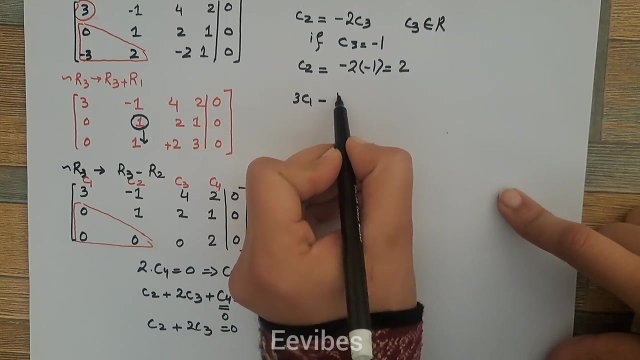 So C2 will be equal to minus 2 times of minus 1, which is equal to 2. fine, Then we will write the last equation from here, which says: 3 times of C1 minus 4, one time or minus. C2 plus 4 times of C3 should be equal to 0. 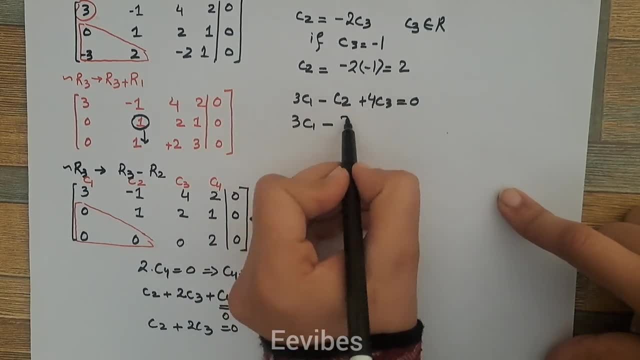 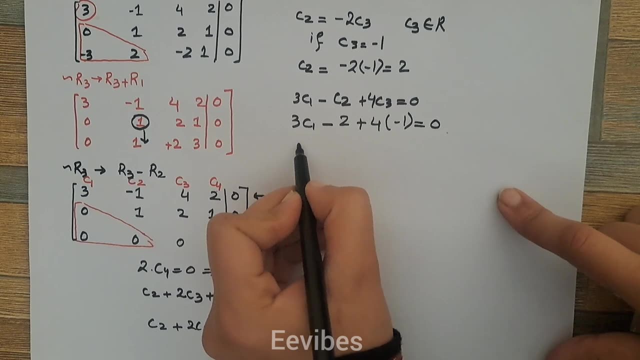 So 3 times of C1 minus C2, which is equal to minus 2 in this case, plus 4 times of C3, which is minus 1, as we selected, and then, on simplification, you will get 3 minus 3C1 minus 2 minus 4 is. 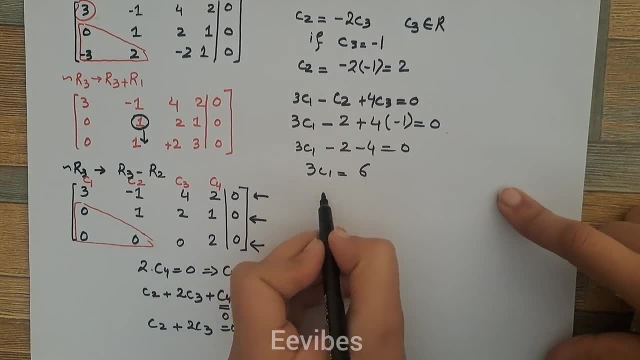 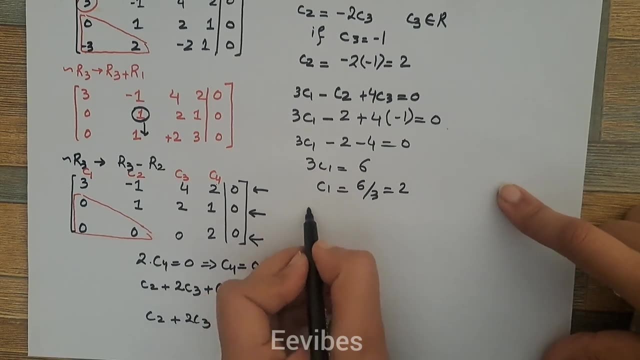 equal to 0, or 3C1 is equal to 6.. C1 will be equal to 6 divided by 3, which is equal to 0. Which is equal to 2.. And hence you can see that the values of the constants are: C1 is equal to 2, C2 is equal.